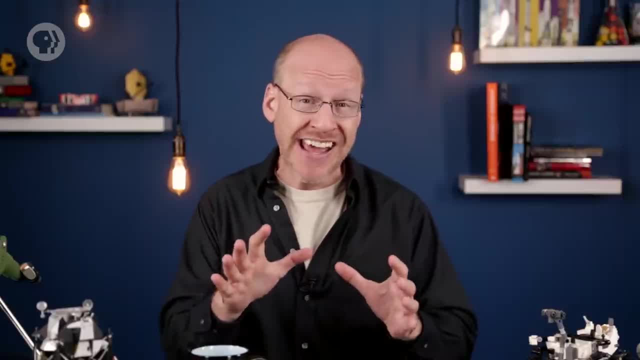 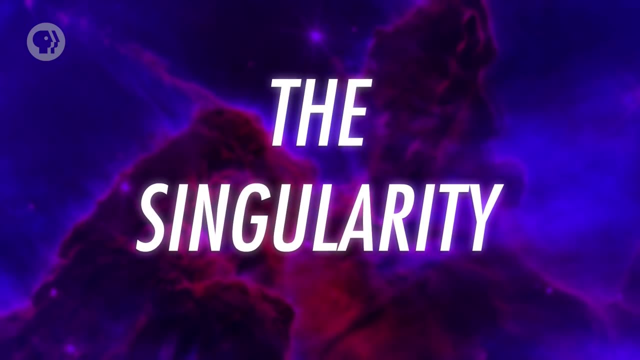 be fairly precise, all of space, time, matter and energy was compressed into a single, infinitely dense point. Astronomers call this the Singularity, which is as good a name as any. Something caused this Singularity to suddenly let loose, expanding violently, cooling and forming. 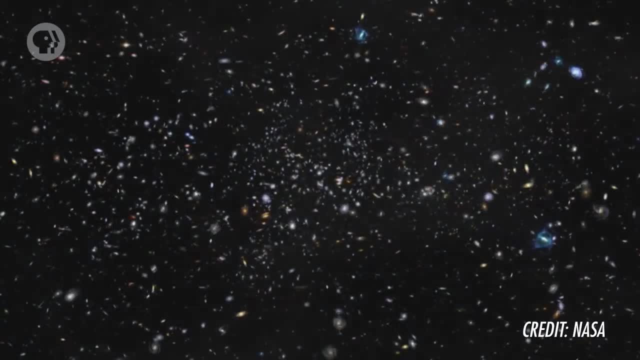 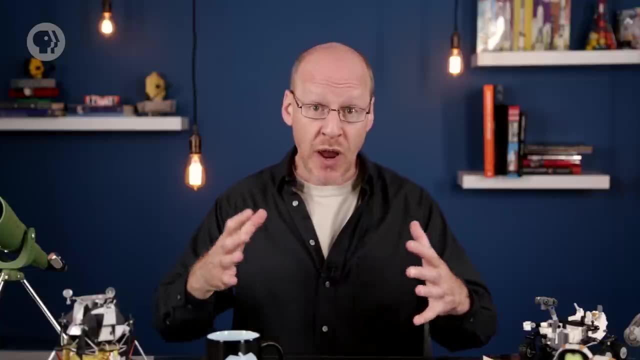 the Universe we see today. Coming to grips with this idea took a while for astronomers, but nowadays the current working model for how the Universe started is with a Big Bang. All the galaxies we see are moving away from each other as space expands between them. That is, on large scales. Remember. 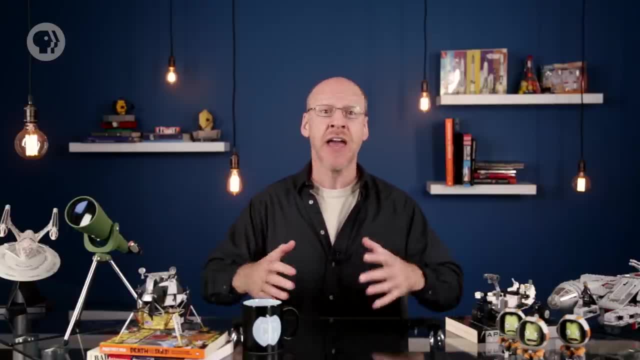 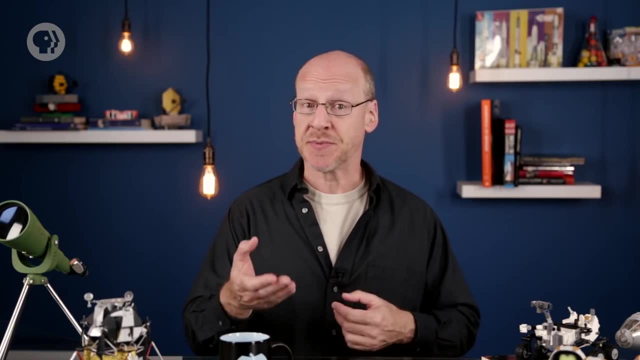 the ruler analogy, where on small scales the expansion is small and on bigger scales the expansion is faster. That's why distant galaxies appear to be rushing away from us fast. On small scales, the expansion is small enough that gravity can overcome it. The Andromeda. 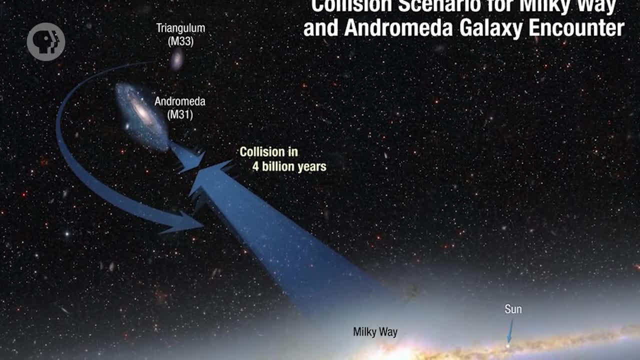 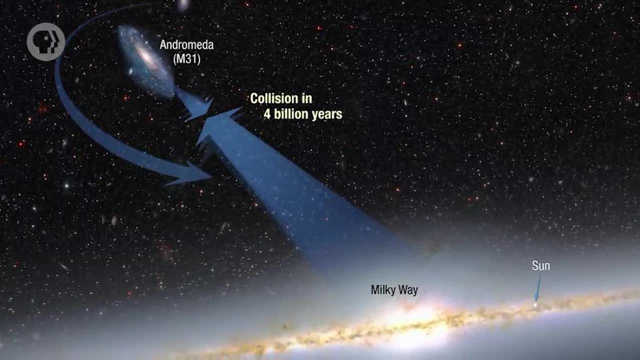 Galaxy, for example, is about 2.5 million light years away. That means it should be moving away from us at about 50 or so kilometers per second, But because of our mutual gravity it's moving toward us. Its motion locally through space is more than enough to overcome. the expansion of space between us. It's like running up the down escalator: Run fast enough and you can make it to the top, But every galaxy has gravity and there are a lot of galaxies in the Universe. That adds up and should affect the expansion of space. It's a lot like the idea of escape velocity: Throw a rock hard enough and even though gravity will slow it down, it will escape. But if you don't throw it fast enough, it'll slow, stop, reverse course and fall back down. 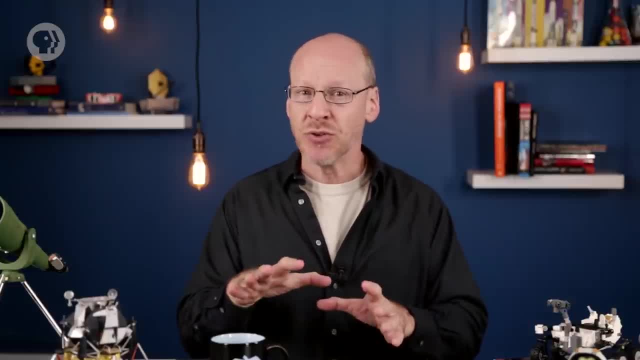 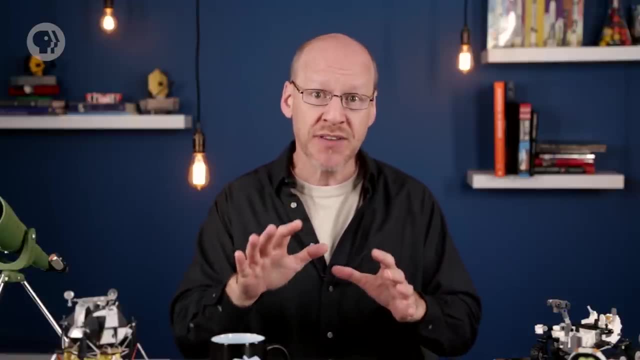 Astronomers fully expected to see this effect on the expansion of space. If you looked on the very largest of scales, you'd expect to see the Universe slowing down, the gravity of the matter in the Universe itself putting the brakes on the expansion And with the 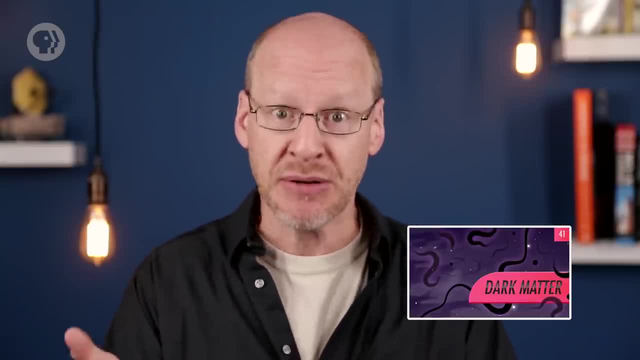 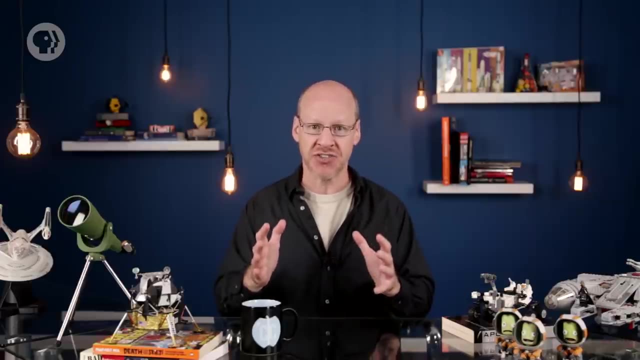 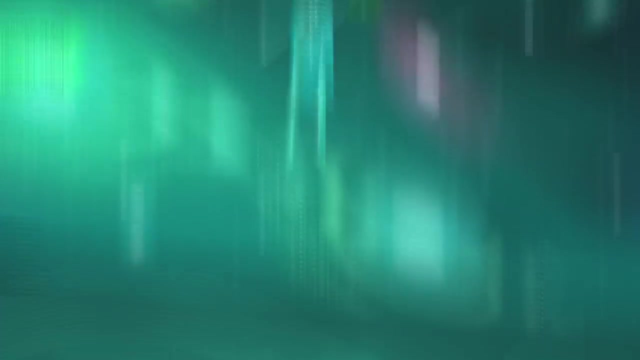 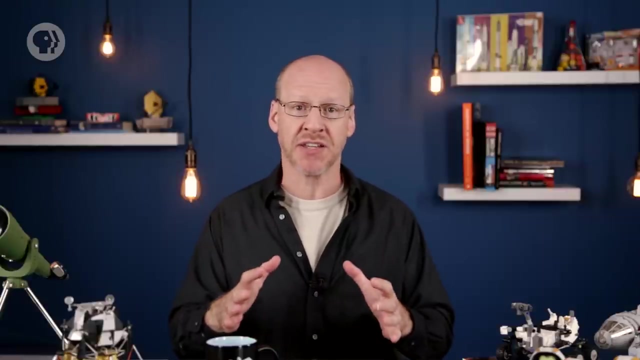 discovery of dark matter. that meant the Universe should be slowing down even more than we first saw. But when astronomers went looking for evidence of this, what they got instead was probably the single biggest shock in the history of astronomy. In the 1990s, two teams of astronomers were using the world's biggest telescopes to 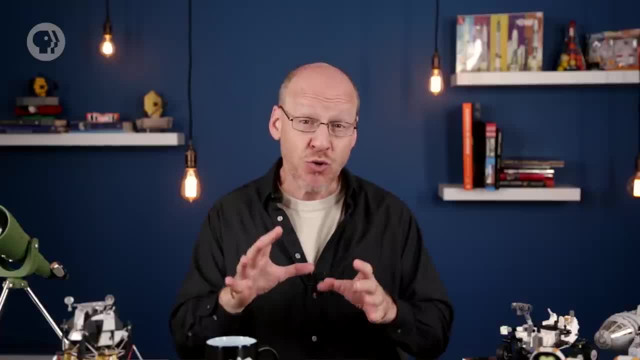 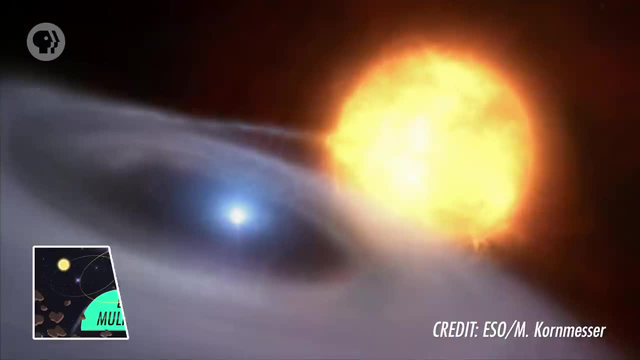 peer as deeply as they could into the Universe. They were looking for incredibly distant supernovae, and not just any kind, but special ones called Type 1a's. these before They occur when a white dwarf increases in mass until electron degeneracy. 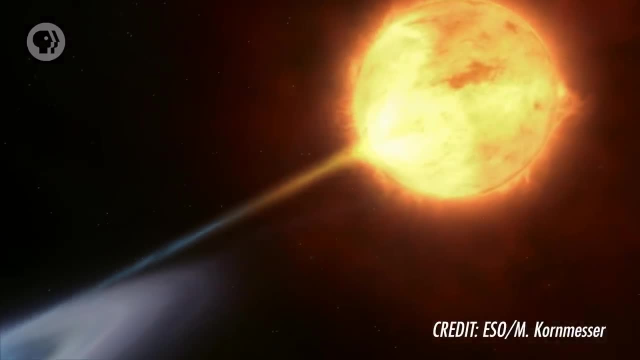 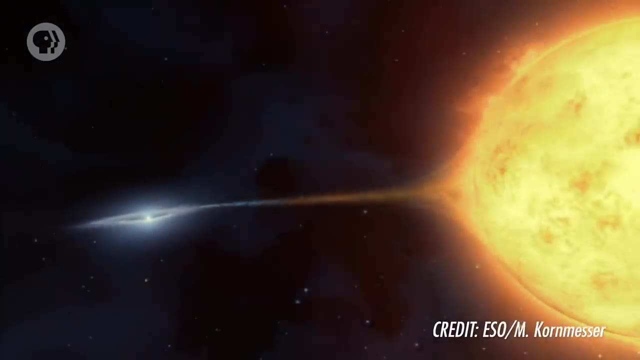 pressure can no longer sustain it against its own gravity, It collapses, undergoes a catastrophic wave of thermonuclear fusion and explodes. The beauty of these types of supernovae is that they all occur. when the mass of the white dwarf gets to about 1.4 times the mass of the Sun, That's the magic number where pressure 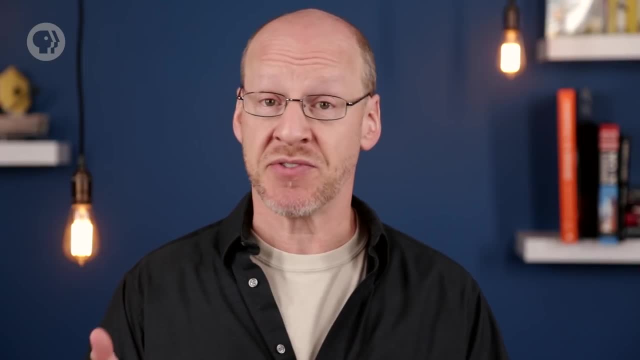 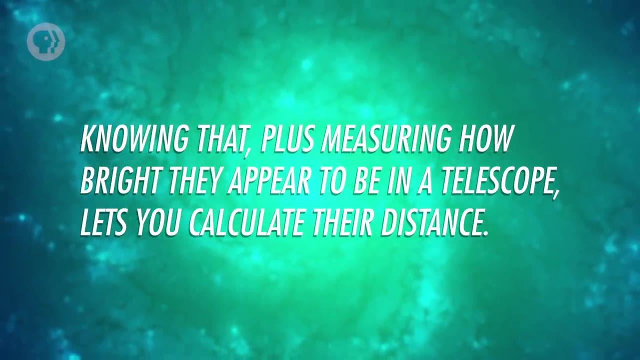 overcomes gravity and they go kablooey. That makes them good standard candles, objects whose intrinsic brightness, whose luminosity is known, Knowing that, plus measuring how bright they appear to be in a telescope lets you calculate their distances. Then those 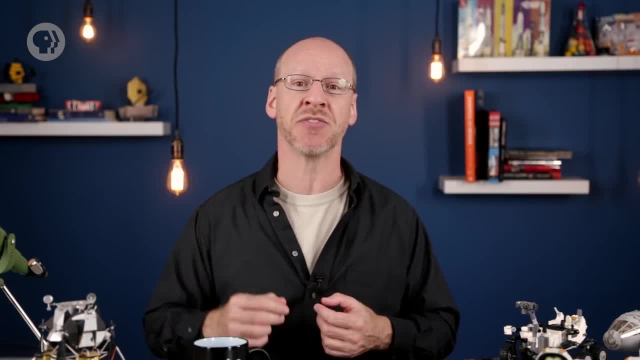 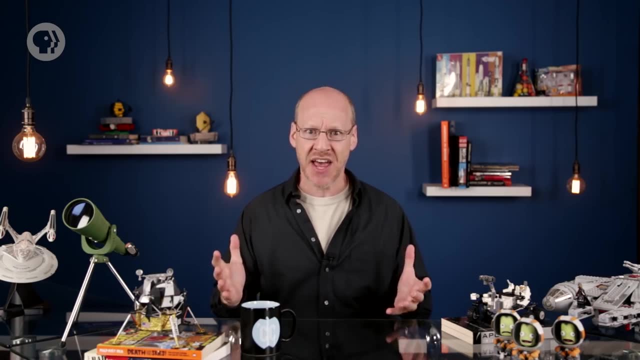 can be compared to the supernovae redshifts, which is a different way of getting their distance. This then tells you how fast the universe is expanding on really big scales. But the results they got didn't make sense. Time and again the supernovae were all fainter. 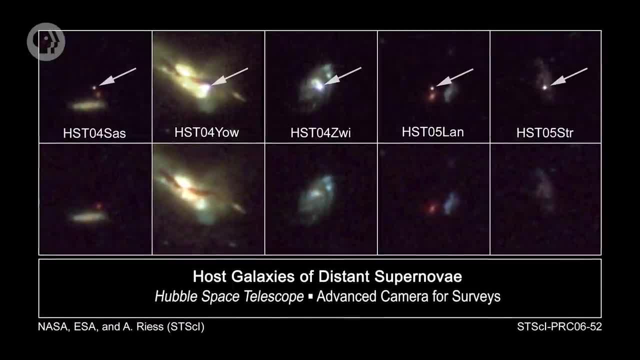 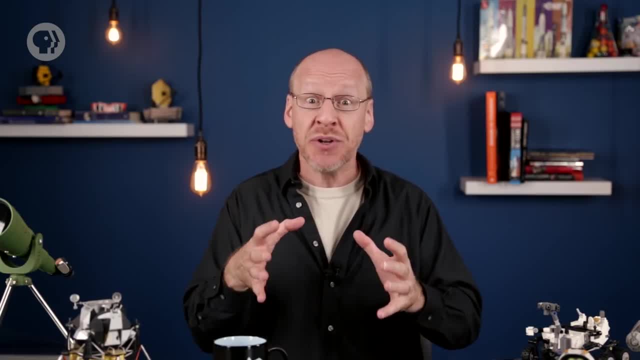 than they expected. It was as if the predictions based on the redshifts were underestimating the distances to the exploding stars. The astronomers did everything they could to see if maybe they had made a mistake somewhere, including making a literal list of things. 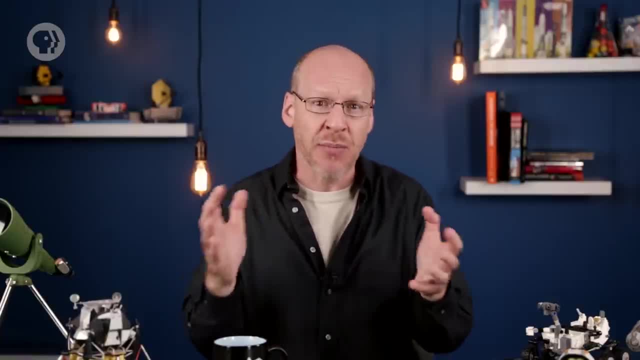 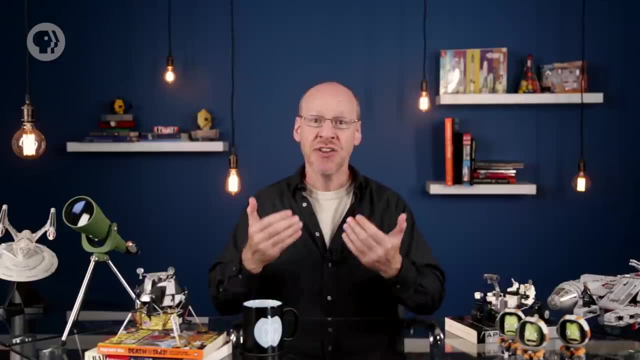 that could make sense. It could make stars look fainter, Intergalactic dust, different chemical compositions for the stars that blew up all kinds of things. But in the end both teams independently came to the same conclusion: The supernovae were. 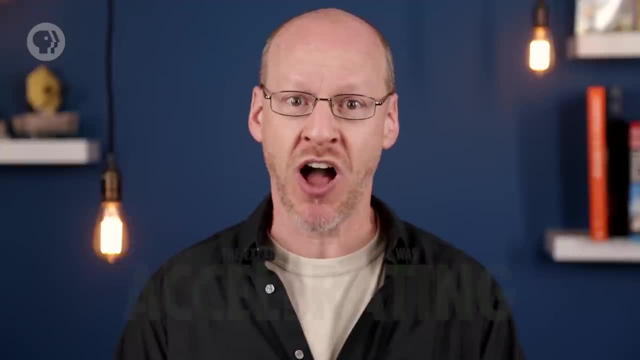 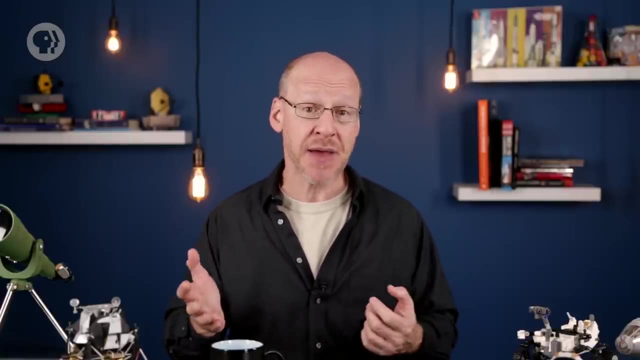 farther away than expected, And that meant something truly shocking: The expansion of the universe was accelerating. Now, remember, that's nuts. We were expecting the expansion of space to be slowing down due to the gravity of all the matter in the universe, But instead 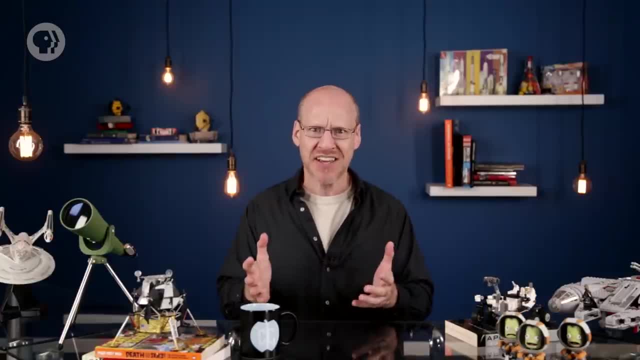 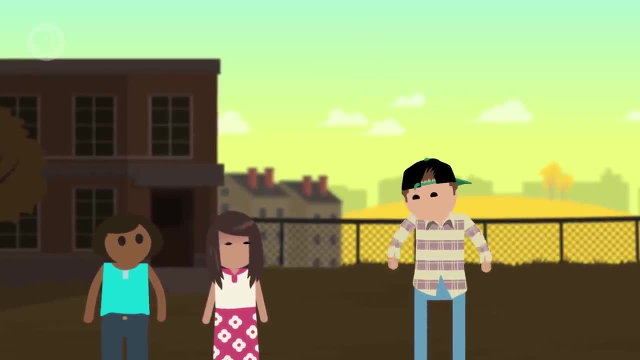 it was speeding up. It's hard to overstate how shocking this is. It's like tossing a rock in the air and instead of it slowing down and falling back down into your hand, it shot upwards faster and faster, defying Earth's gravity. 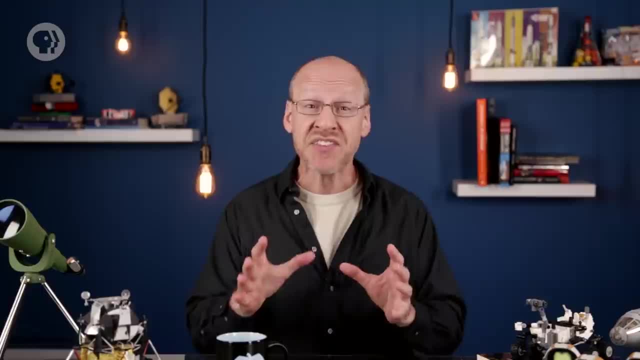 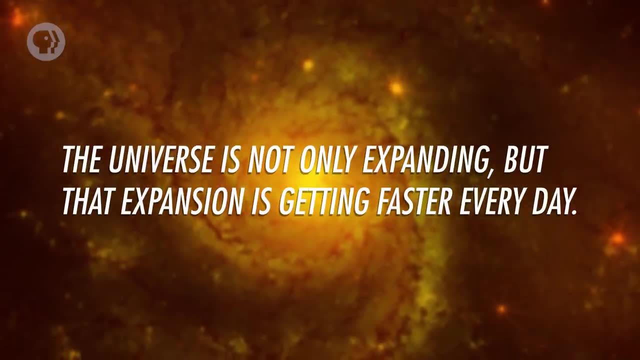 Of course scientists were skeptical, Many still are, But in the end, several other independent measurements have verified this result. The universe is not only expanding, but that expansion is getting faster every day. What could possibly cause such a thing? To be flatly honest, we don't know, Well not. 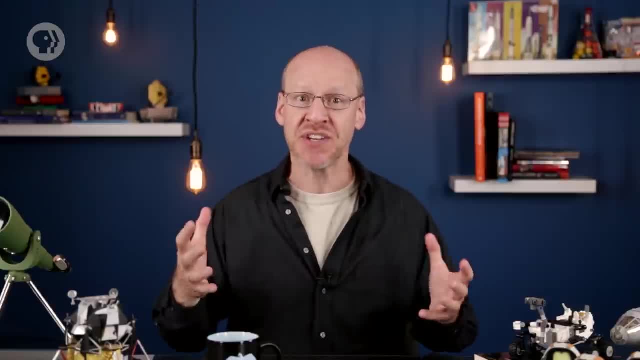 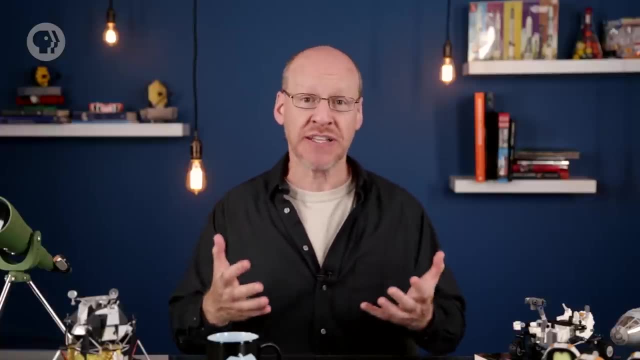 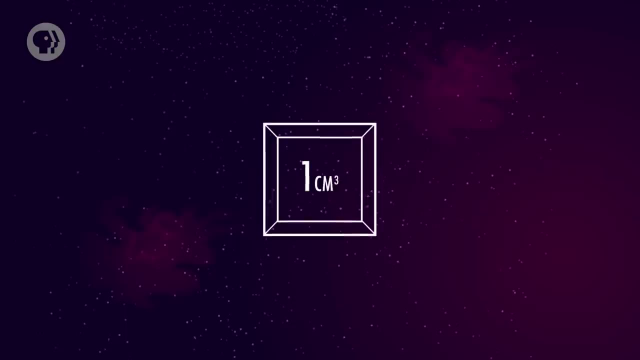 exactly, But whatever it is acts like an energy suffusing space pushing the universe into motion, And we can't see it, so it's invisible. We already have dark matter, so naturally this got tagged dark energy. It seems to be a property of space itself, a tiny bit of energy in every single cubic. 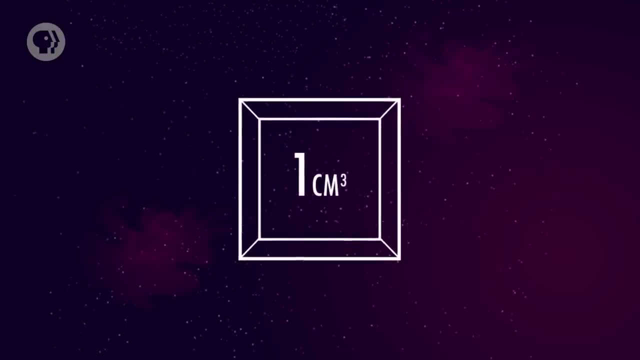 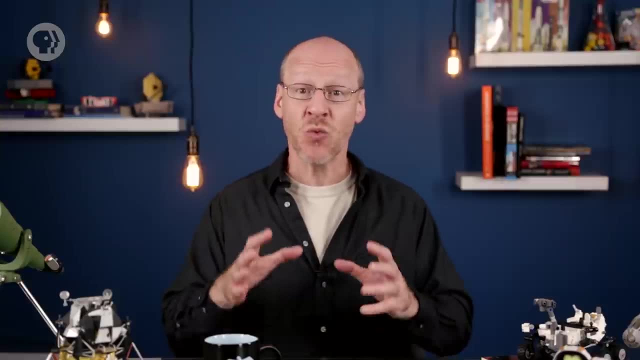 centimeter of the universe. The amount per cc is incredibly small, But there are a lot of cubic centimeters in the universe. It adds up And we can add it up. Now that we have measurements of this, we can take an inventory of the universe. We can total all of the matter. 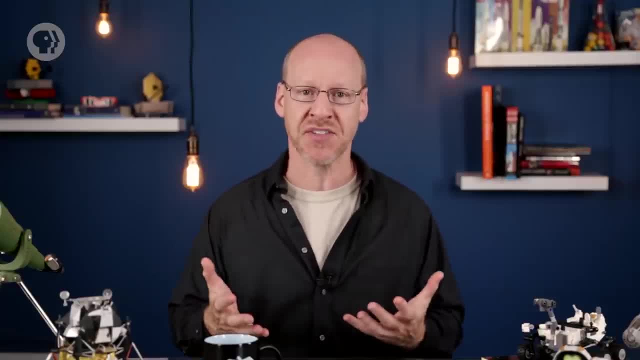 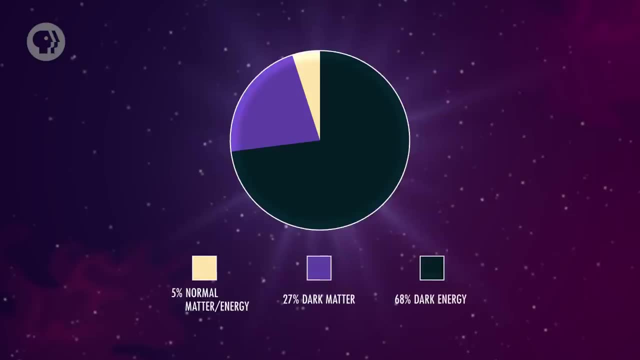 and energy. there is making a sort of budget of stuff in the cosmos. When we do, it looks like this: 95% of the universe is made of stuff we can't directly see. Normal matter is outnumbered 20 to 1.. Maybe we should rethink calling it normal. 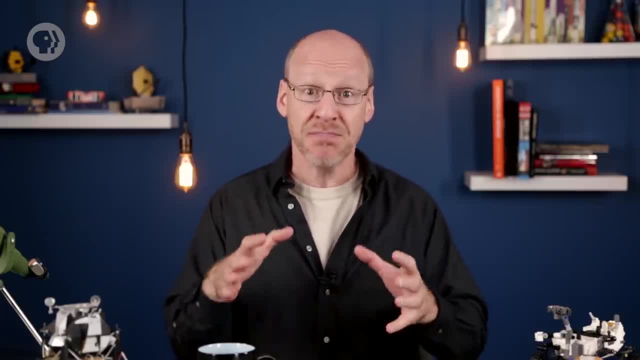 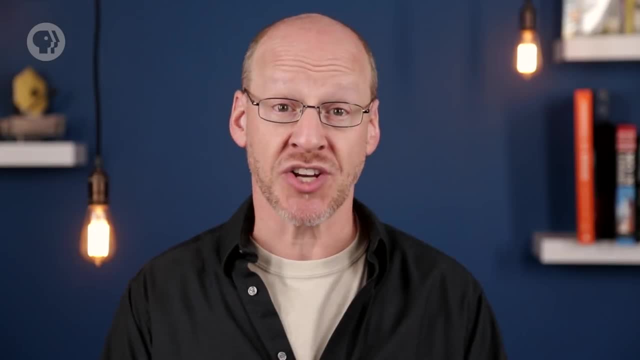 So if two-thirds of the cosmic budget is made up of dark energy, it must have some pretty big effects, right Yeah, like changing the eventual fate of the entire universe. A big question. one of the biggest is: will the universe expand forever? 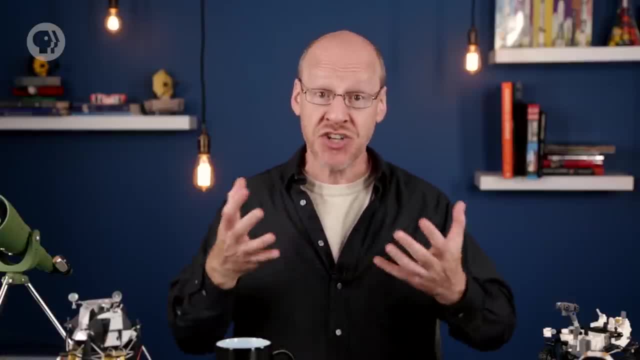 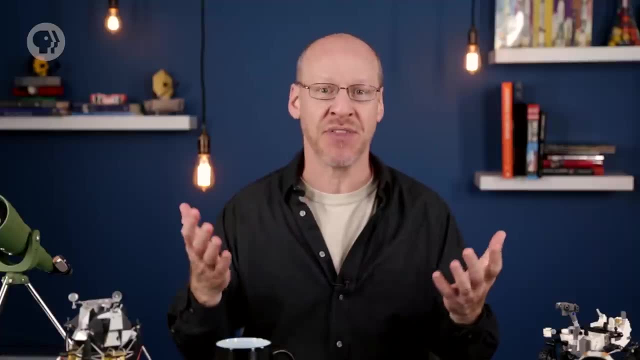 Well, astronomers have a framework to answer this question. We call it the geometry of the universe. Matter has gravity and gravity bends space. So is there enough matter in the universe to stop the expansion? The geometry of the universe mathematically describes its overall curvature, the shape of space on the. 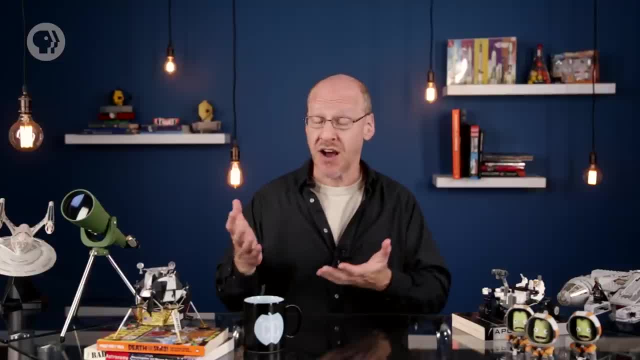 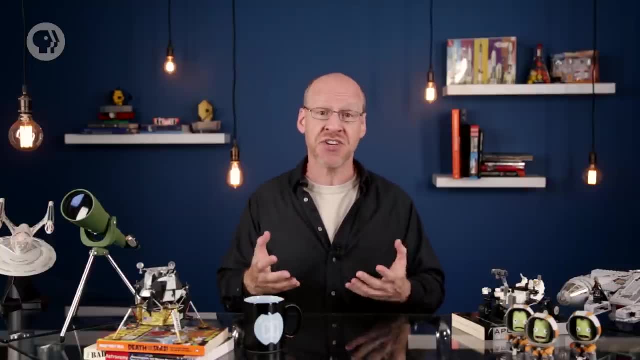 largest scales of all. To be clear, this concept is important to cosmologists, but it can be weird and confusing to someone who is just learning about all this. Still, a lot of astronomy classes teach it, so I'm going to go over it very briefly And, if you want more information, 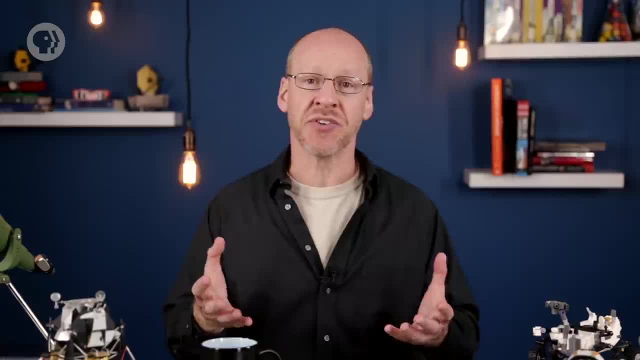 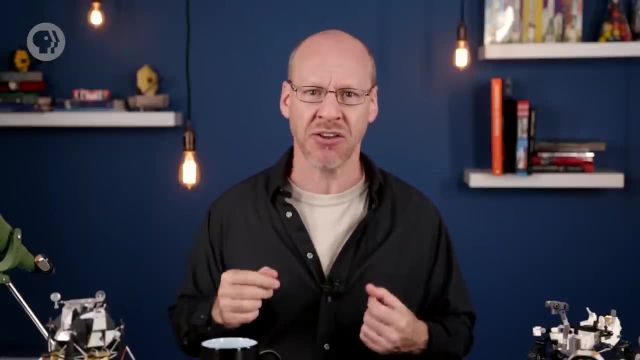 we have links in the doobly-doo. The idea behind the geometry of the universe is that if there's enough matter, the cosmic expansion will slow, stop, and then everything will re-collapse, a sort of big bang in reverse. If there's not enough matter, then the universe will expand forever, And in between the two, 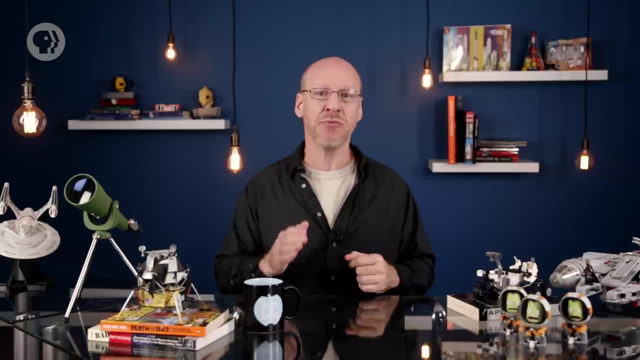 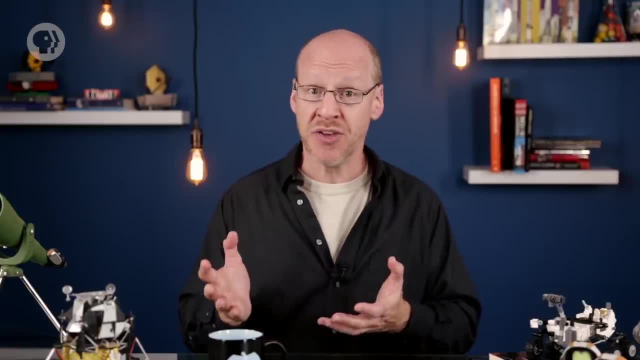 there's just enough matter that the expansion slows but never quite reaches zero until an infinite amount of time in the future. Conceptually it's a lot like escape velocity. It was once thought that the geometry of the universe, tied to the amount of matter in it, determined its destiny. But don't get. 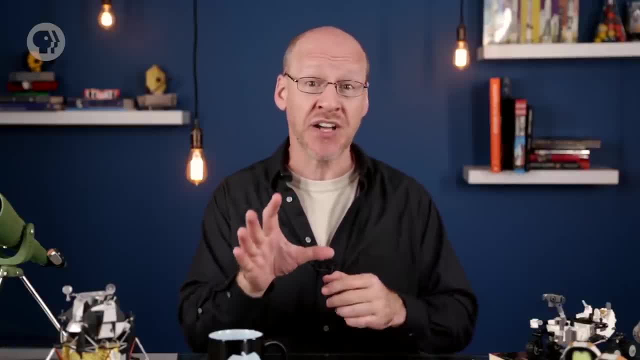 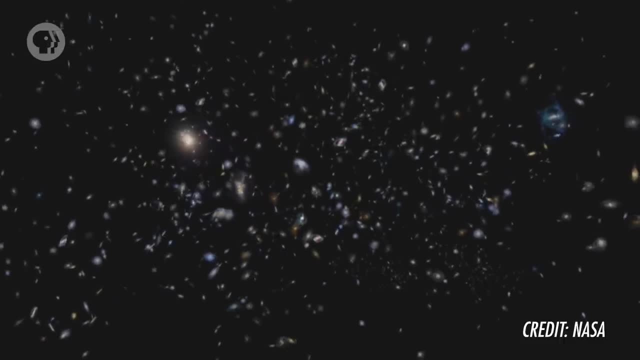 me wrong. dark energy threw a monkey in the wrench for that, and geometry alone doesn't determine the eventual fate of the cosmos. We think there's enough dark energy in space to ensure the expansion will continue forever, despite the geometry. Dark energy is just. 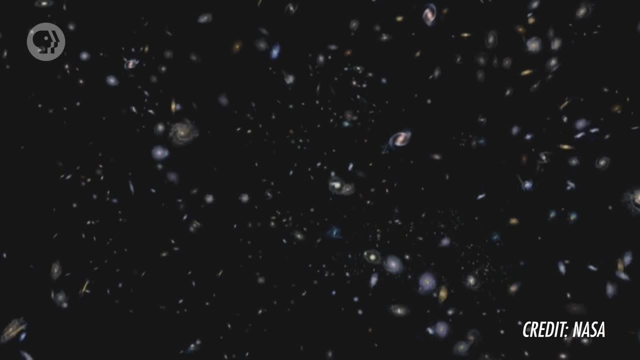 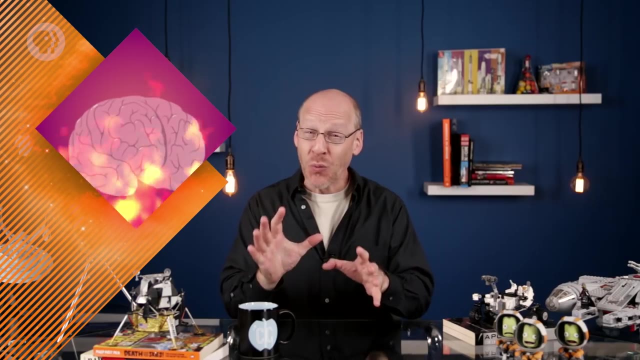 too powerful and will always drive the expansion of the universe ever faster. So for now, the answer, as far as we can see, is yes, the universe will expand forever. OK, there's one more brain-melty thing we need to talk about For this part, you might. 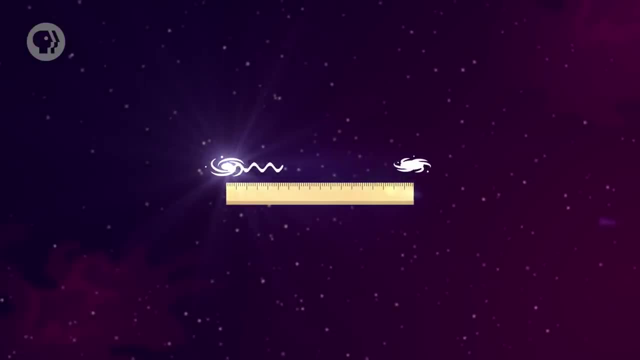 want to sit down. Space itself is expanding As light travels from one galaxy to the next. it fights that expansion, losing energy, just like you use up energy climbing a staircase. When light loses energy, its wavelength gets longer. That's what cosmological redshift is The 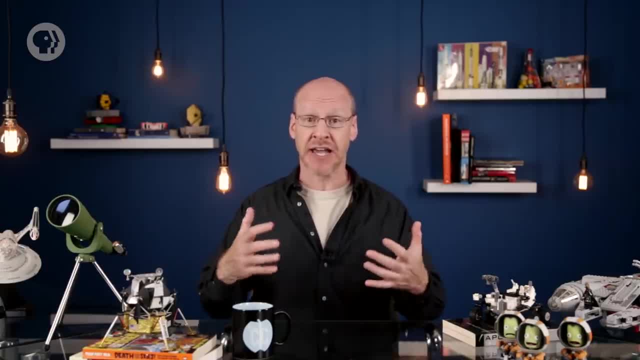 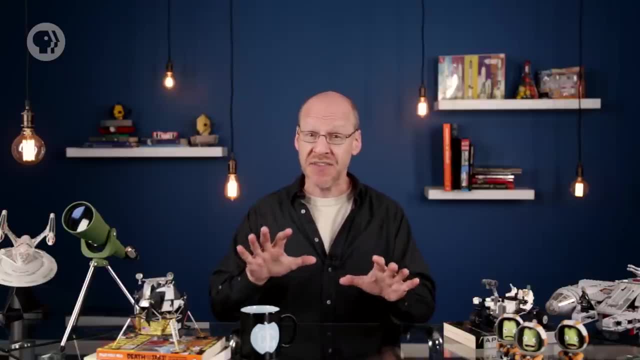 more distant the galaxy, the faster it recedes and the more energy light loses as it travels to us. But wait, At some distance from us, space would be expanding so quickly that a galaxy in that part of the universe would be moving away from us at the speed of light. 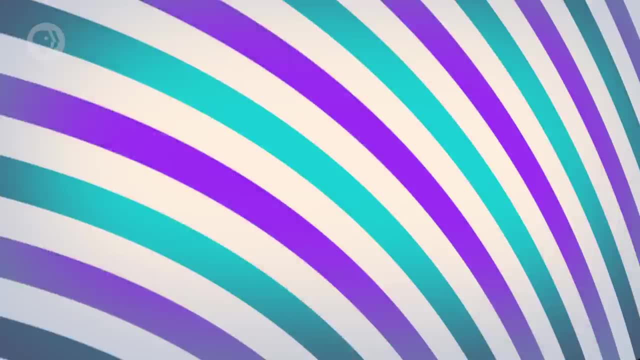 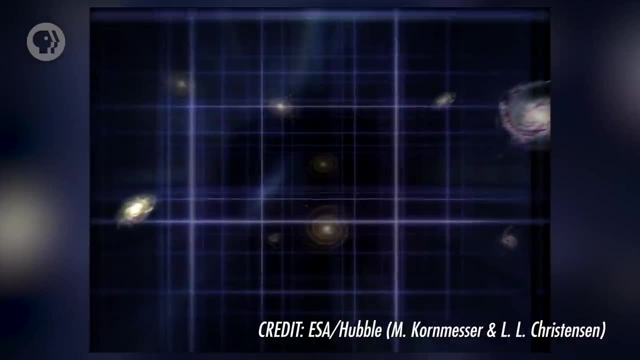 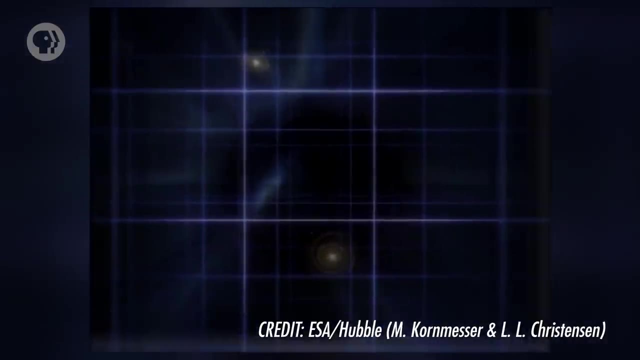 Moving farther away would be swept away from us faster than light. Now, before you start complaining: yes, this is possible. The speed of light is the ultimate speed limit in the universe if you're traveling through space, But space itself is exempt from that rule. It can expand at whatever speed it wants. The matter in it: galaxies. 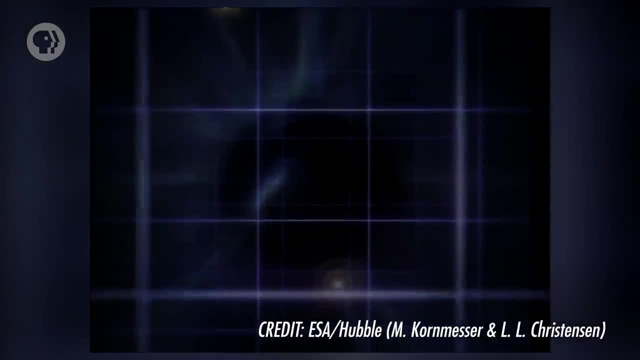 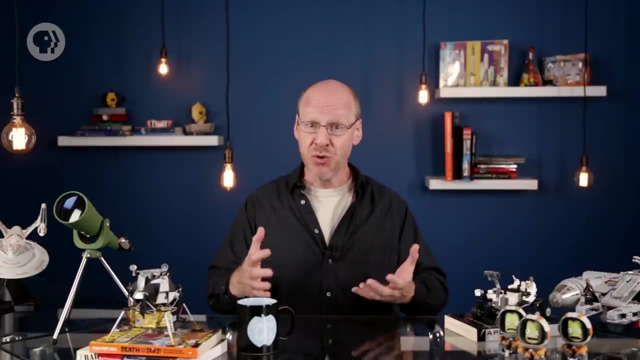 stars and such is swept along with it, so they're not traveling so much through space as with it. When you solve the equations to calculate distance in redshift, the distance a galaxy would have to be from us to be moving away at the speed of light. 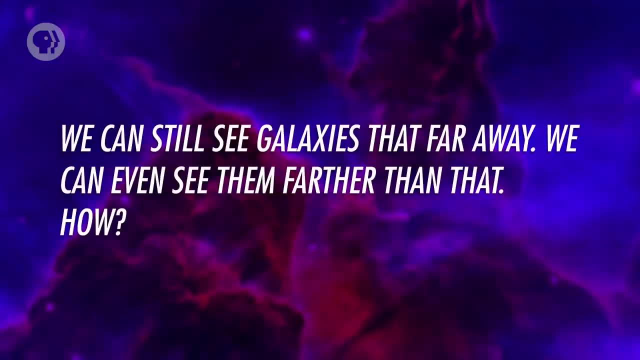 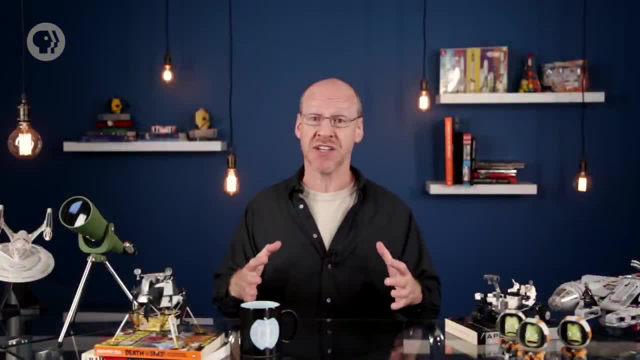 is about 13.8 billion light years. Here's the fun thing: We can still see galaxies that far away. We can even see them farther than that. How? It's? because that distance is how far the galaxy is from us. now, When? 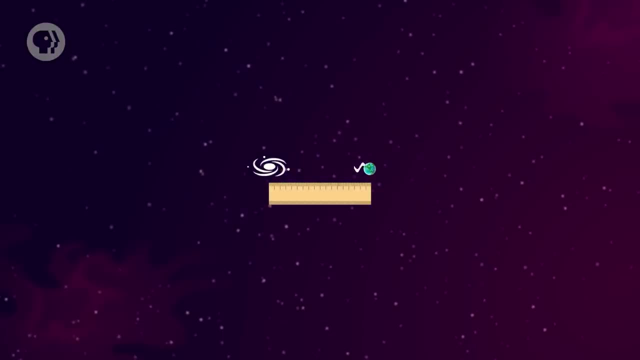 it emitted that light, the universe was much younger, smaller and the galaxy closer to us. It would have been about 4.5 billion light years away at the time, and the light took over 9 billion years to get here. Back then, the space between us and the galaxy wasn't. expanding as rapidly so the light could keep pace At that time. the space between us and that galaxy means we're moving away from each other at light speed, But back then we were close enough to see each other. For that same reason, we can see galaxies that are moving away from us faster than light. because when they emitted that light, there was less space separating us. The most distant galaxies we see are now about 45 billion light years from us. We call this the radius of the observable universe. It's essentially the cosmic horizon. Mind you, the actual universe may be far larger than this. Who knows, maybe even infinite. 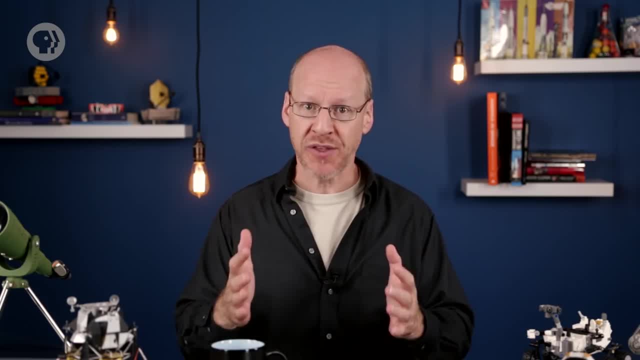 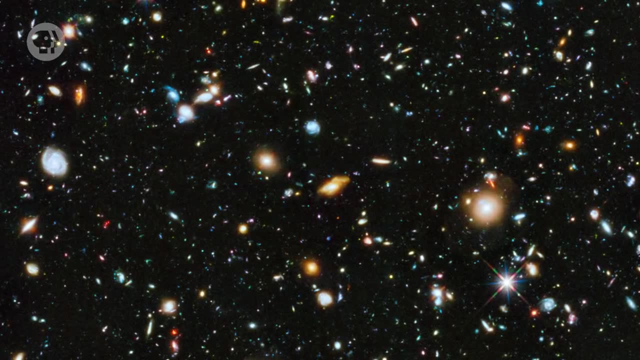 But we can only see galaxies that are by now 45 billion light years away. That's our horizon. If space were simply expanding, the size of the observable universe would expand as well. But we have dark energy and space expands more rapidly every day. That means a truly 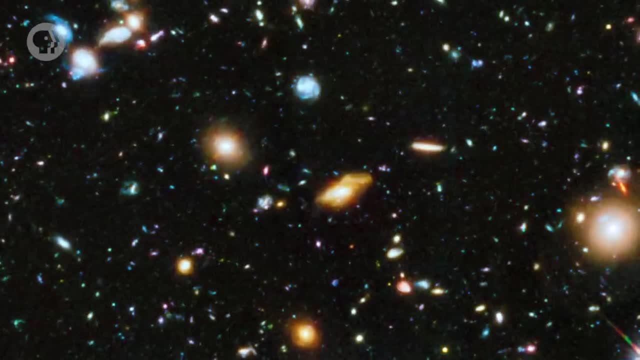 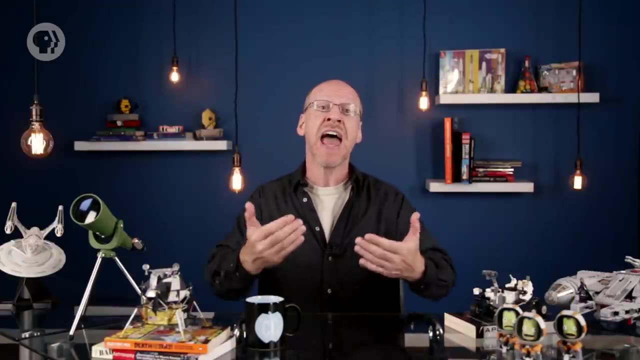 distant galaxy's light is fighting more and more expansion all the time. It's like climbing an ever-steepening staircase, Compared to a constant expansion. a galaxy in an accelerating universe has to be closer for us to see it. It's losing energy faster.